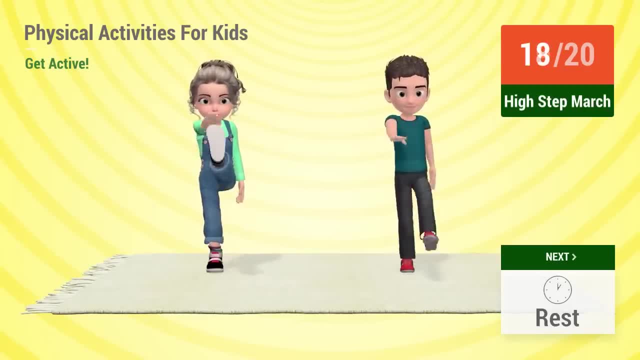 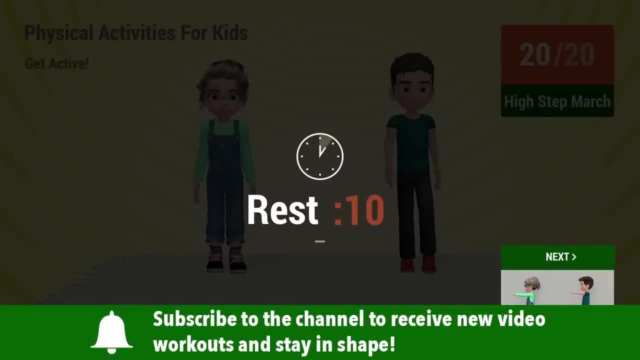 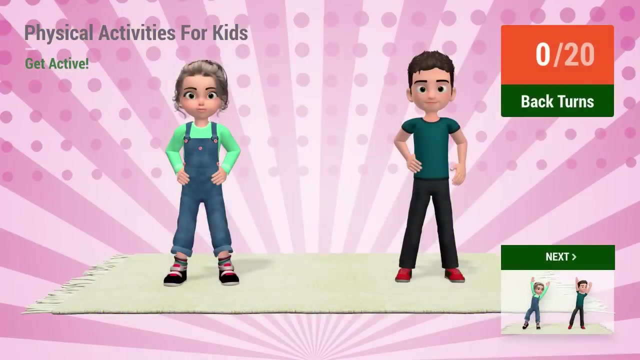 19, 20.. Rest time. Up next back turns In 5,, 4,, 3,, 2,, 1, go 1,, 2,, 3,, 4,, 5,, 6,, 7,, 8,, 9,, 10,, 11,, 12,, 13,, 14,, 15,, 16,, 17, 18.. 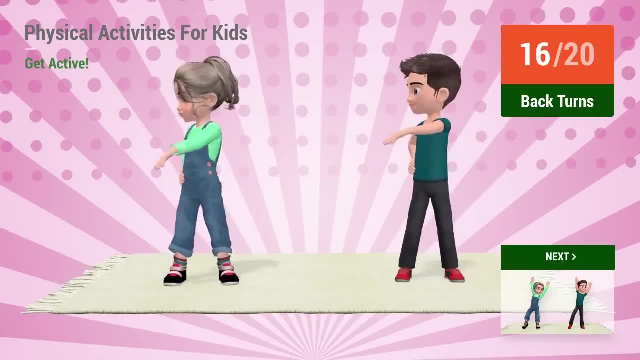 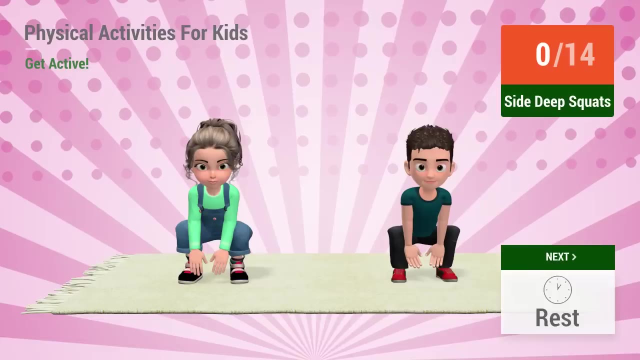 19, 20.. Up next side deep squats In 5,, 4,, 3,, 2,, 1, go 1,, 2,, 3,, 4,, 5,, 6,, 7,, 8,, 9,, 10,, 11,, 12,, 13,, 14,, 15,, 16,, 17,, 18,, 19,, 20.. Up next high knee jacks In 5,, 4,, 3,, 2,, 1, go 1,, 2,, 3,, 4,, 5,, 6,, 7,, 8,, 9,, 10,, 11,, 12,, 13,, 14,, 15,, 16,, 17,, 18,, 19, 20.. 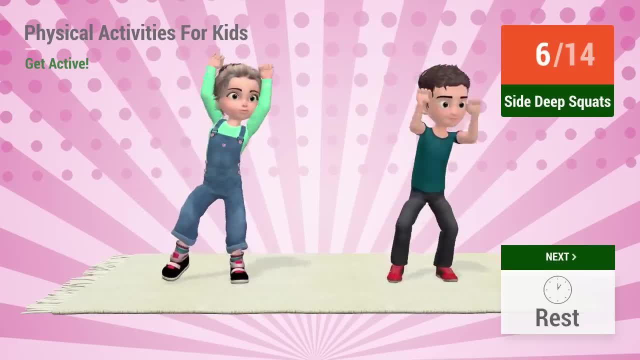 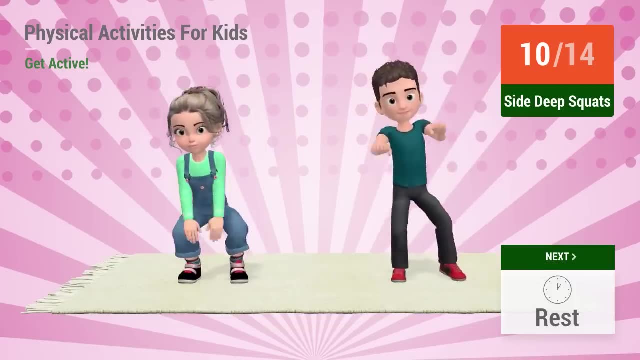 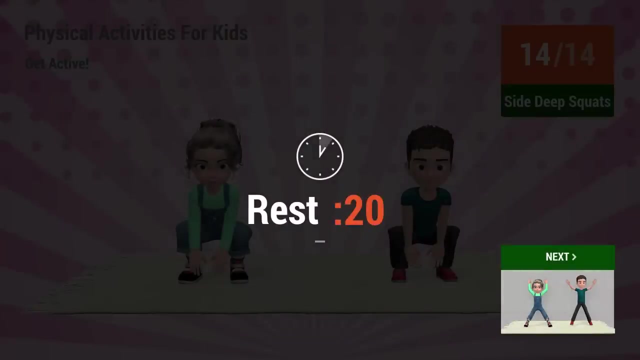 15., 6., 7., 8., 9., 10., 11., 12., 13., 14.. Rest time: From the beginning: Rest time: Congratulations, You've passed the three-minute mark. Keep working out. Let's see how far you can go. 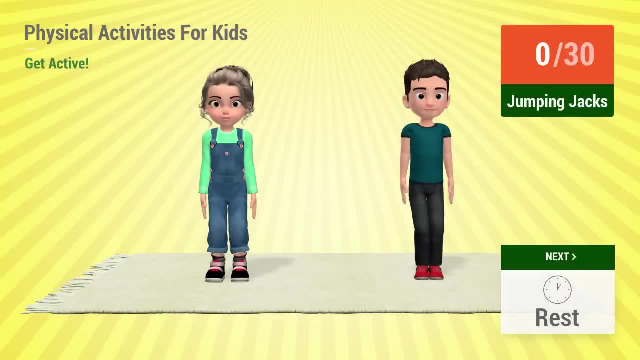 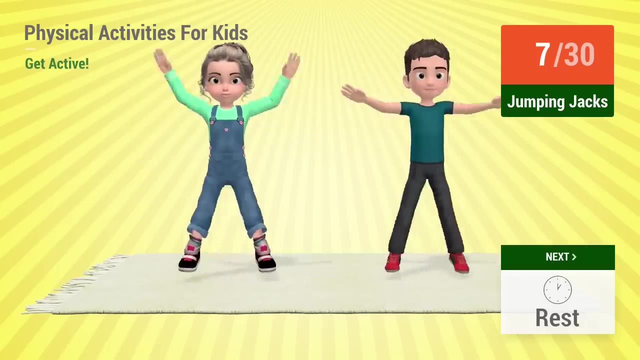 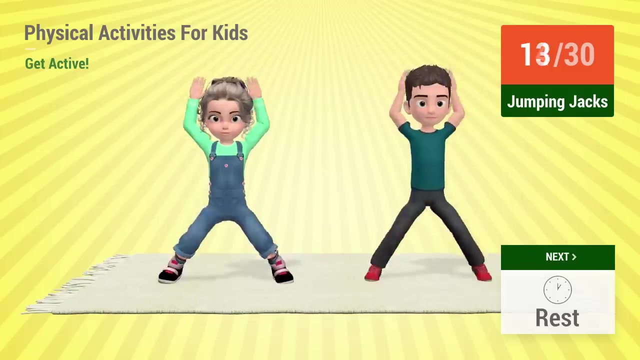 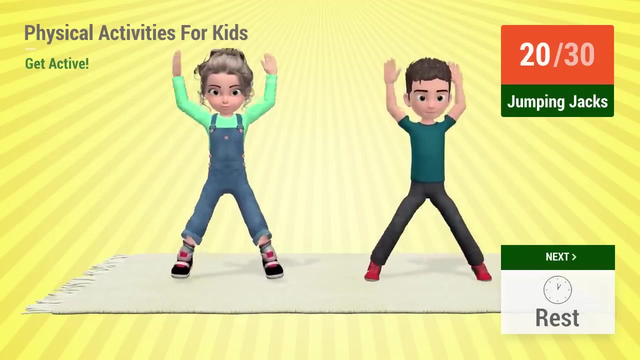 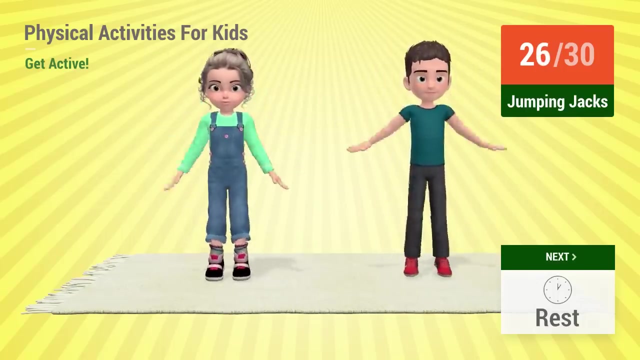 Up next jumping jacks In 5,, 4,, 3,, 2,, 1, go 1,, 2,, 3,, 4,, 5,, 6,, 7,, 8,, 9,, 10,, 11,, 12,, 13,, 14,, 15,, 16,, 17,, 18,, 19,, 20,, 21,, 22,, 23,, 24,, 25,, 26,. 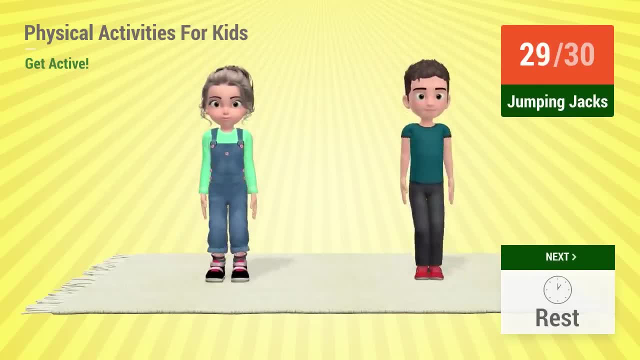 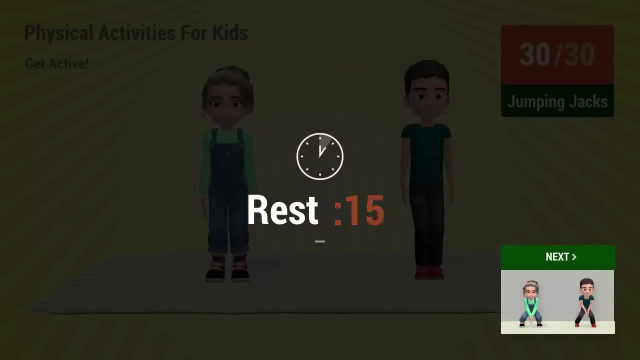 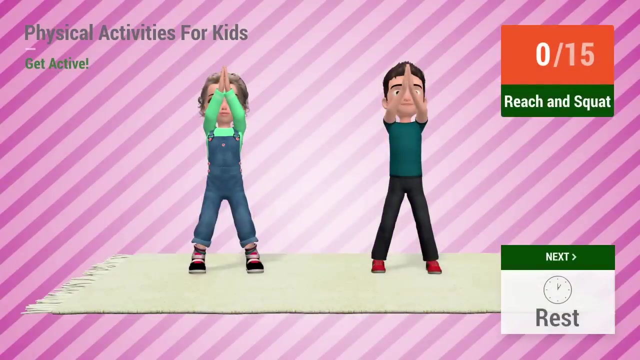 27,, 28,, 29,, 30. Rest time- Rest time. Up next, reach and squat In 5, 5,, 4, 3, 2, 1, go 1, 2,. 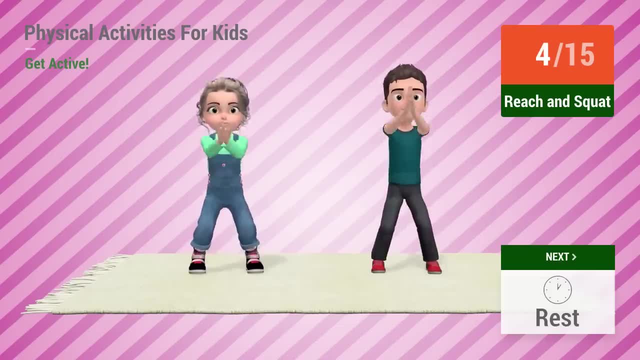 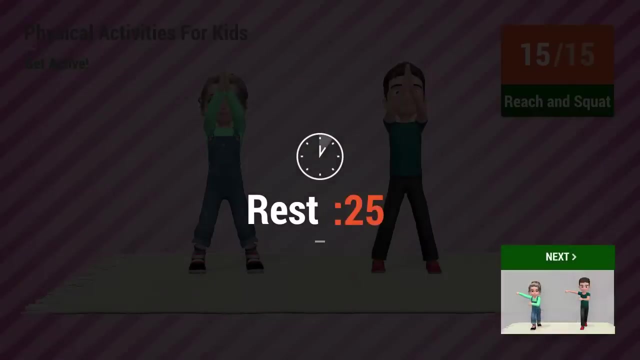 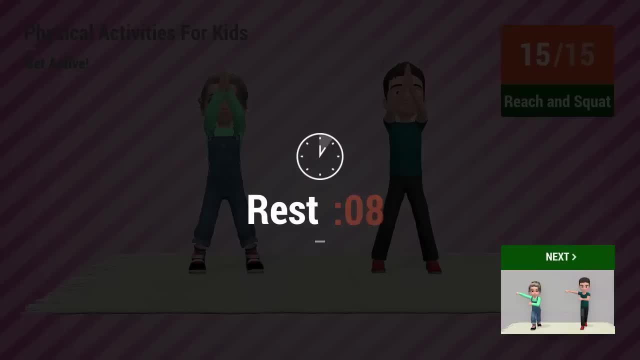 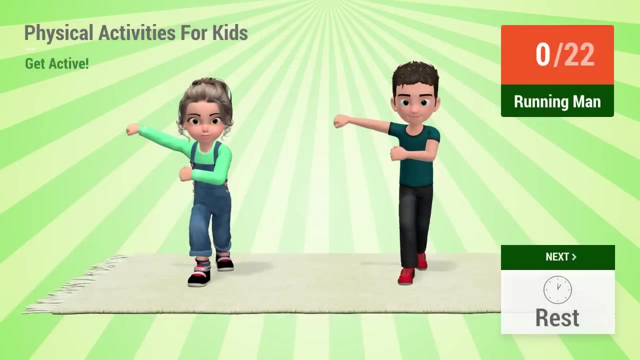 45 left, 45,, 55,, 56,, 57,, 58,, 59,, 58,, 60,, 62,, 62,, 62,, 63,, 63,, 64,, 63, Up next Running Man in 5,, 4,, 3,, 2,, 1, go. 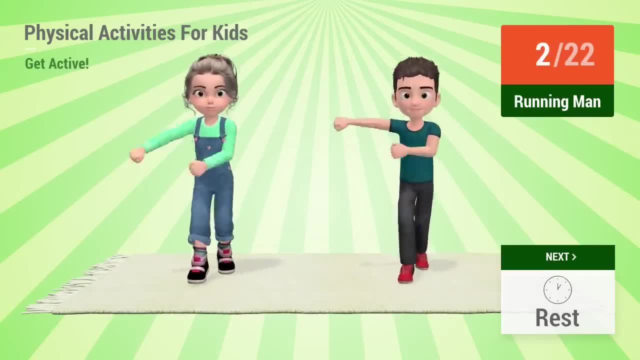 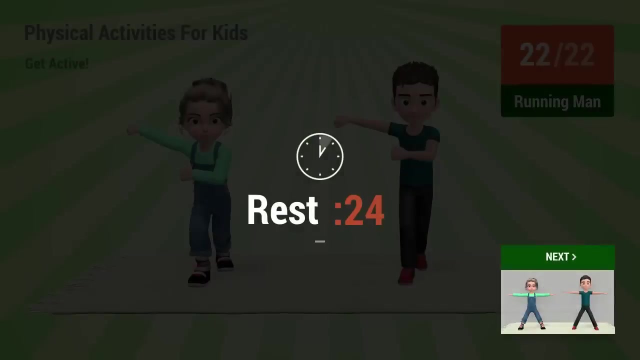 5,, 6,, 7,, 8,, 9,, 10,, 11,, 12,, 13,, 14,, 15,, 16,, 17,, 18,, 19,, 20,, 21,, 22, rest time. 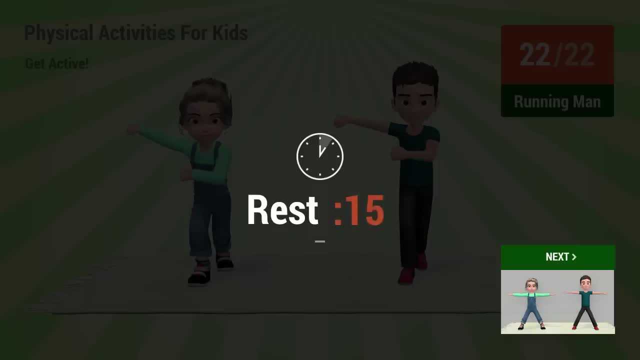 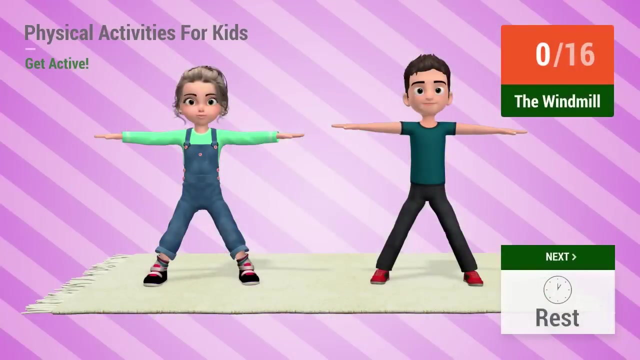 Up next The Windmill in 5,, 4,, 3,, 2,, 1, go 1,, 2,, 3,, 4,, 5,, 6,, 7,, 8,, 9,, 10,, 11,, 12,, 13,, 14,, 15,, 16,, 17,, 18,, 19,, 20,, 21,, 22,. rest time. 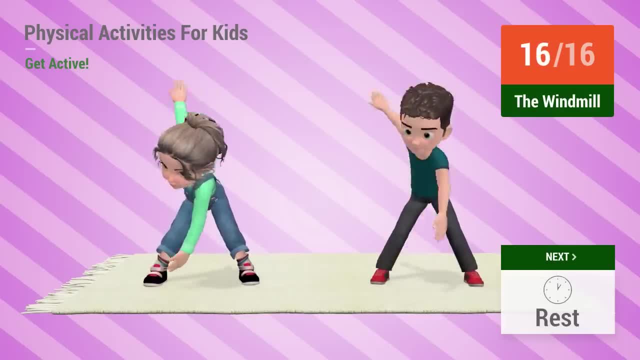 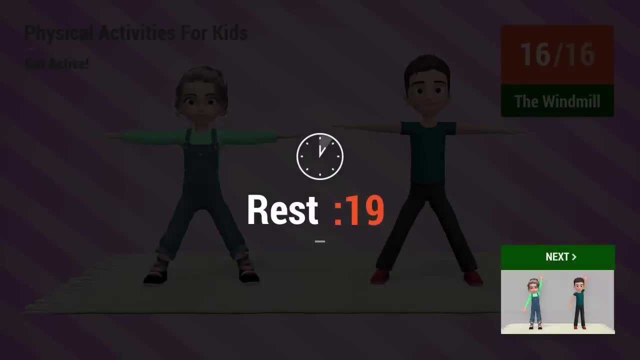 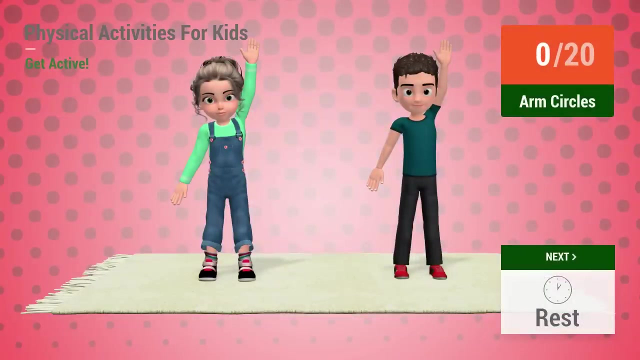 15, 16, rest time. Up next Arm Circle in 5,, 4,, 3,, 2, 1, go 1,, 2,, 3,, 4,, 5,, 6,, 7,, 8,, 9,, 10,, 11,, 12,, 13,, 14,, 15,, 16,, 17,, 18,, 19,, 20,, 21,, 22, rest time. 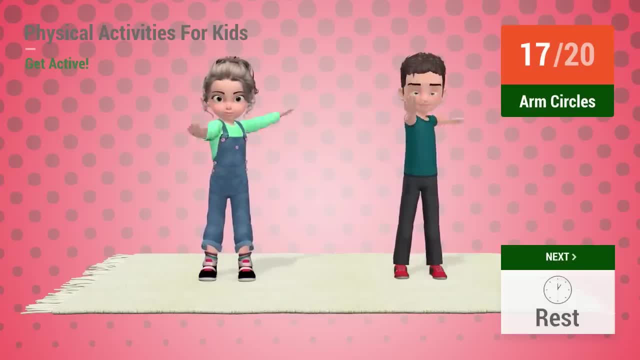 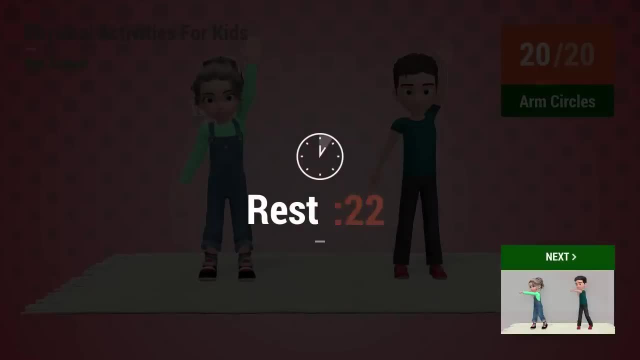 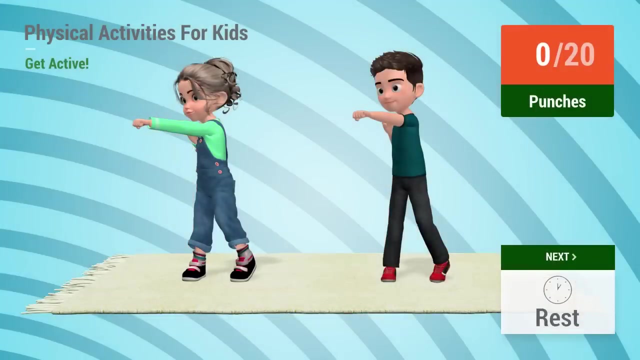 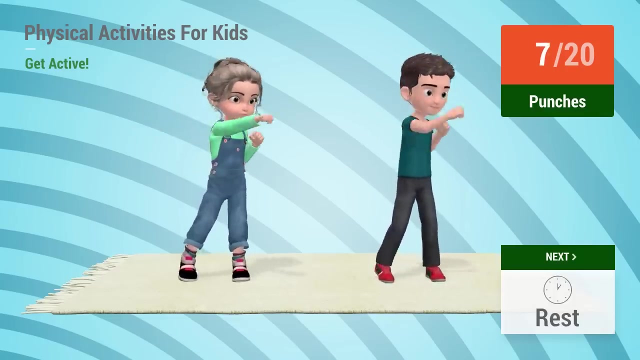 16,, 17,, 18,, 19,, 20, rest time. Up next Punches in: 5,, 4,, 3,, 2,, 1, go 1,, 2,, 3,, 4,, 5,, 6,, 7,, 8,, 9,, 10,, 11,, 12,, 13,, 14,, 15,, 16,, 17,, 18,, 19,, 20,, 21,, 22, rest time. 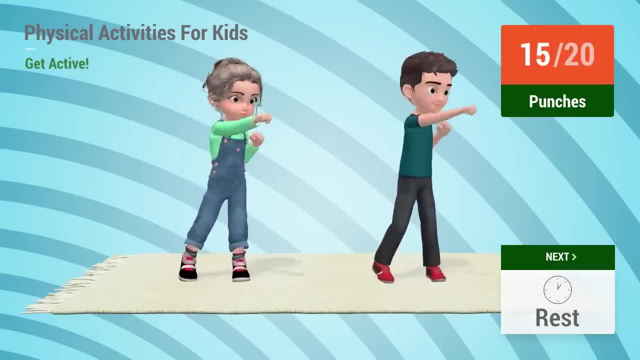 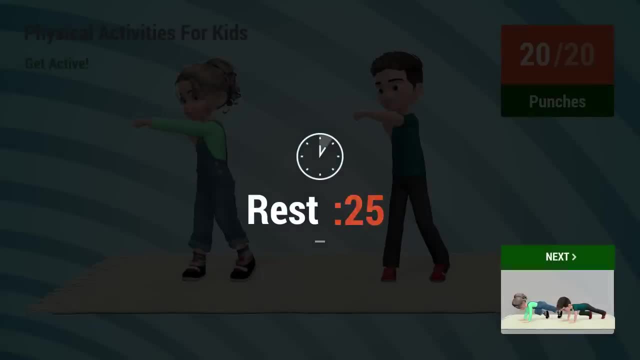 1,, 2,, 3,, 4,, 5,, 6,, 7,, 8,, 9,, 10,, 11,, 12,, 13,, 14,, 15,, 16,, 17,, 18,, 19,, 20, rest time. 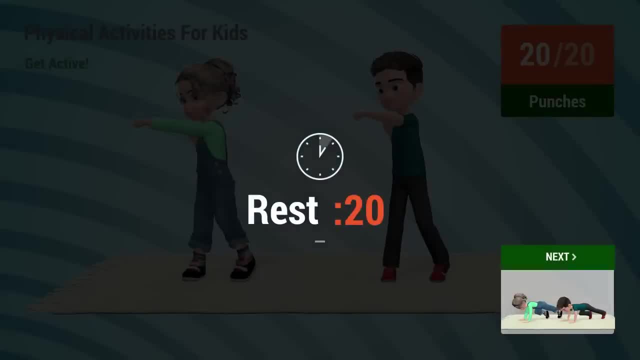 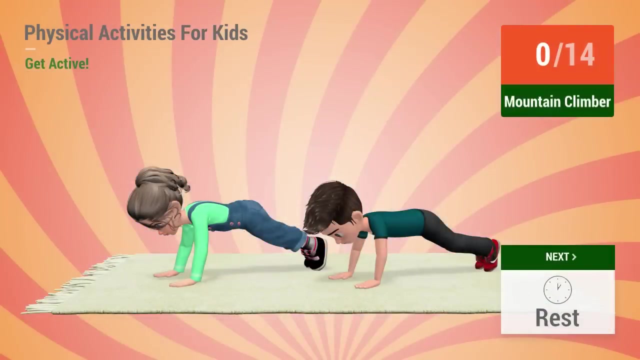 1,, 2,, 3,, 4,, 5,, 6,, 7,, 8,, 9,, 10,, 12,, 13,, 18,, 19,, 20, rest time Up next Mountain Climber in 5,, 4,, 3,, 2,, 1, go. 1,, 2,, 3,, 4,, 5,, 6,, 7,, 8,, 9,, 10,, 11,, 12,, 13,, 16,, 18,, 19,, 20,, 20,, 16,, 20,, 21,, 23,, 24,, 23,.